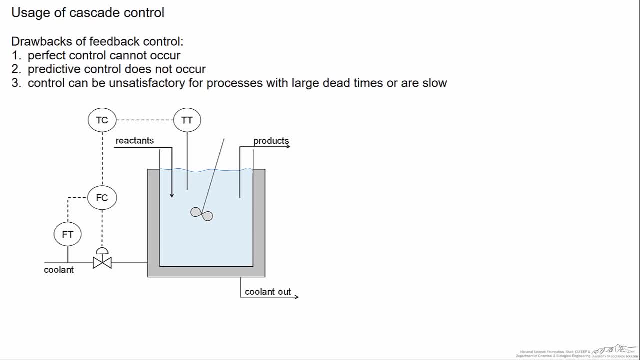 perfect control cannot occur. This may or may not be of huge concern, but it does work out more conveniently if you can develop a process where for a particular disturbance, it can handle the disturbance such that the controlled variable is not changed. The second issue: 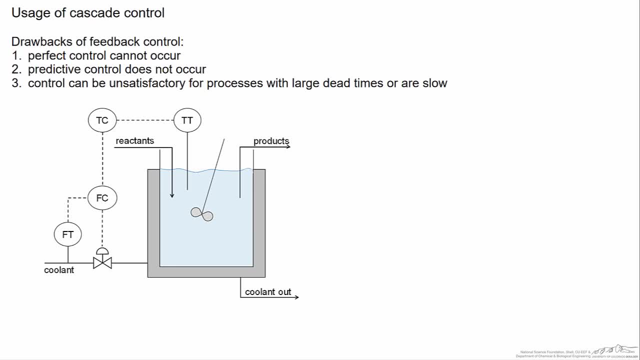 is that predictive control does not occur with a feedback only scheme. Why? Because remember what feedback control does? Feedback control only deals with measurements of the controlled variable. So therefore, even if we knew something was going to happen, like we knew that there was going to be a flow rate change somewhere in the process, a temperature, 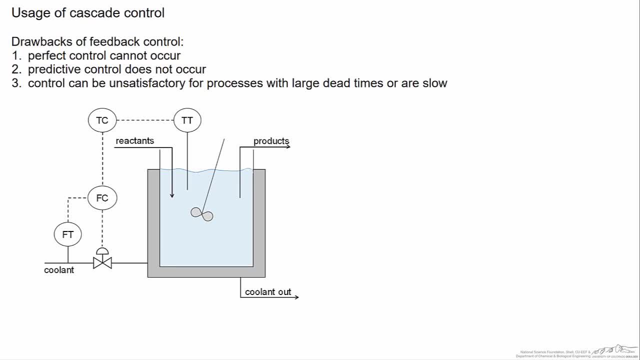 change a pressure, change something along those lines, the feedback control scheme will not occur. scheme will not be able to handle that until there is a deviation in the value of the controlled variable. So therefore, for processes which have heavy disturbances having a feedback, 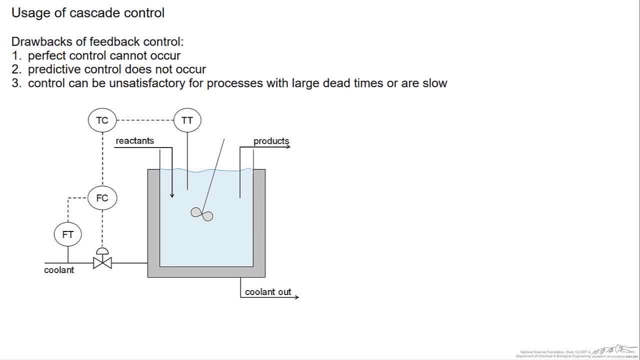 only scheme may have some problems And related to that is for processes which are very slow or have large dead times. they don't necessarily handle disturbance as well because of that slow time to respond. So a disturbance will happen, but because of the large dead time. 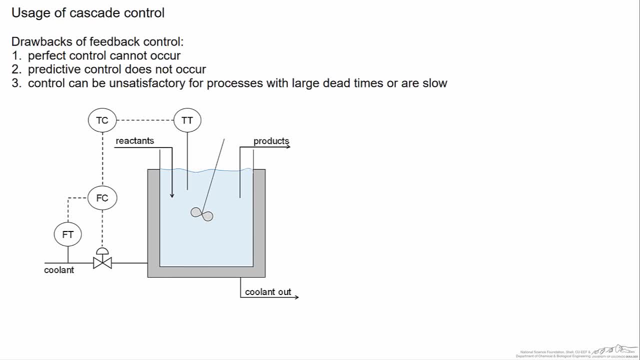 of the process or large tau value, the time constant of the process- it will not be able to handle disturbances in a very efficient, quick manner, leaving the process away from its steady state for a lengthy period of time. So cascade control cannot provide perfect 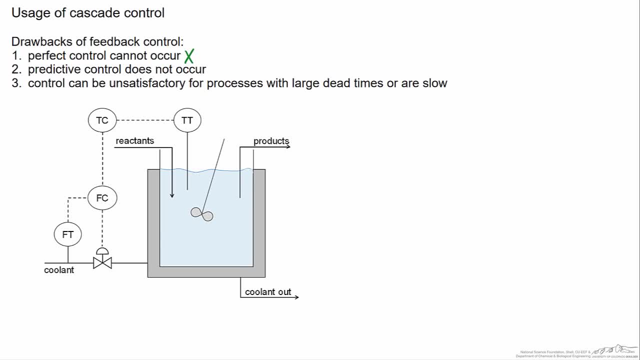 control. we'll discuss why a little bit later on. however, it can help with both predictive control and speeding up the process. both of those two are directly related to each other, So cascade control can be handled by a very efficient, quick manner, leaving the process. 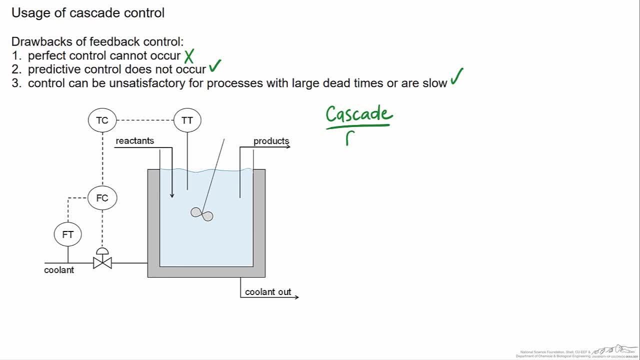 smooth and smooth. So, for instance, a reaction to the current speed control can best be approximated as the idea of feedback. control loops in series, And to exemplify this we have a jacket reactor on the diagram where the desired variable to control here is the temperature inside. 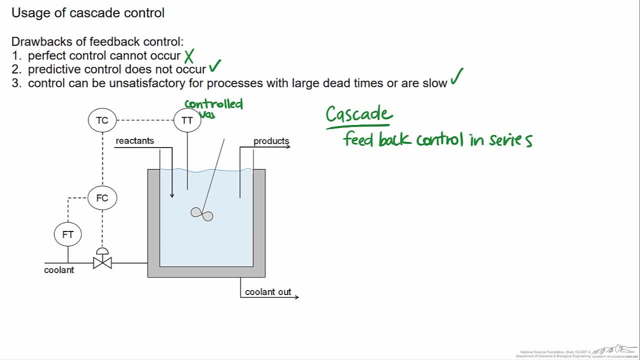 the reactor. so this is our controlled variable, and the reason why you'd want to control temperature in a reactor would be that it can be useful to prevent runaway reactions. it can also be a nice way to, based on doing a mass balance on the systems, control the temperature in. 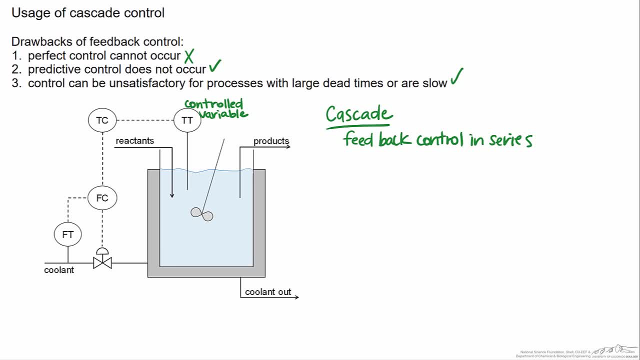 balance on the system, know what your products are going to be. so, therefore, to get your system at its desired output, You have to set a particular temperature, because temperature dictates reaction rate. So in this control scheme, the manipulated variable is going to be the flow rate of coolant to the system. Obviously, there's a whole host of other ways. 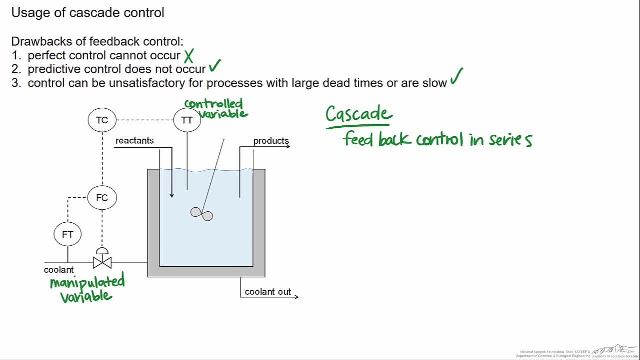 in which this could be manipulated, but for the sake of what we're doing here, it's the flow rate of the coolant. The temperature controller does not directly connect to the valve. There is a second layer here where the temperature controller sends its signal. 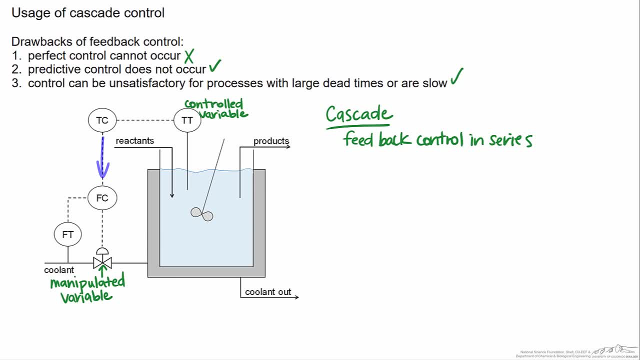 to a flow controller, and then the flow controller is also taking information from the flow rate of the coolant. So what it's measuring here is the coolant flow rate, and the flow controller is taking that information in addition to the information from the temperature controller. 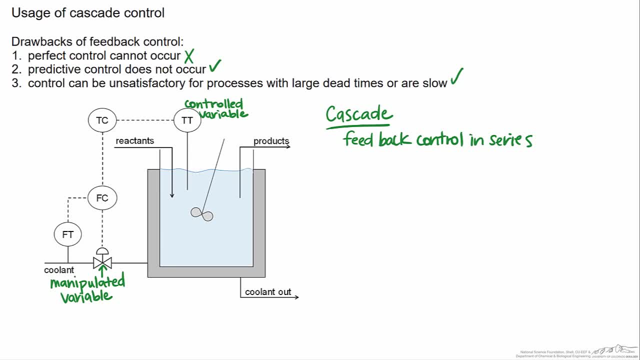 in order to adjust the valve. So the temperature controller is represented as the primary control controller. The primary controller in a cascade control scheme will always be the control that corresponds to the controlled variable, in this case the reactor temperature and the flow controller is the secondary controller. Primary, secondary, there can be more than. 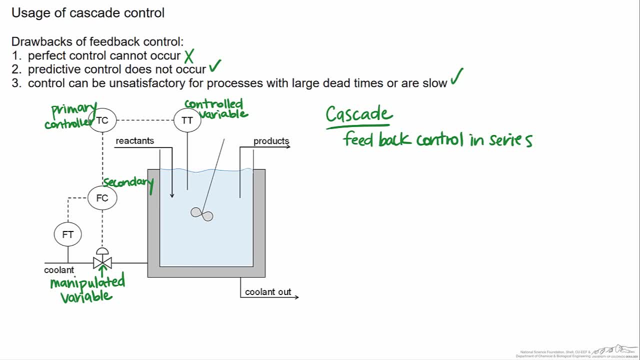 two layers of cascade control, so it can be ternary, quaternary, etc. Whatever is lowest in the hierarchy is the one that will directly control the valve. Important information about the secondary control. there are two things that need to be the case in order for this to be a useful cascade control scheme. The first is the variable. 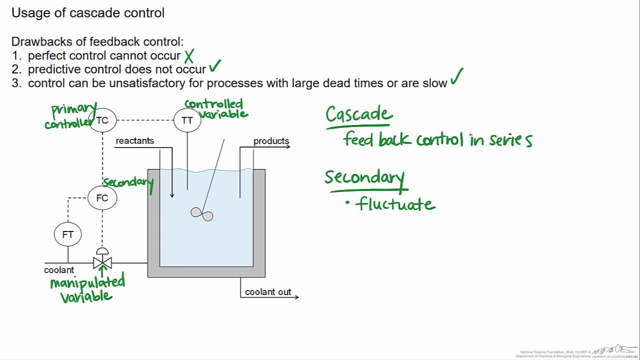 must fluctuate and it must be a non-negligible fluctuation. Why? Because if the variable doesn't fluctuate, then the extra information being provided to the process is not useful. Additionally, if the fluctuations are relatively small in scale- and small is in the eye of 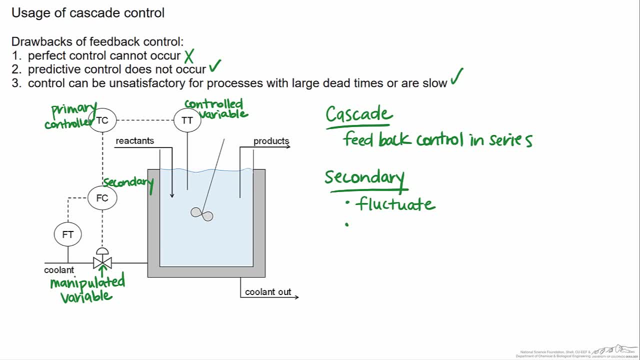 the beholder, then again it really is a problem. It really isn't going to help improve this process. The second part is remember that the whole idea of cascade control- if we look at the disadvantages of feedback control- is to speed up the process response. So therefore the secondary control loop must have a faster 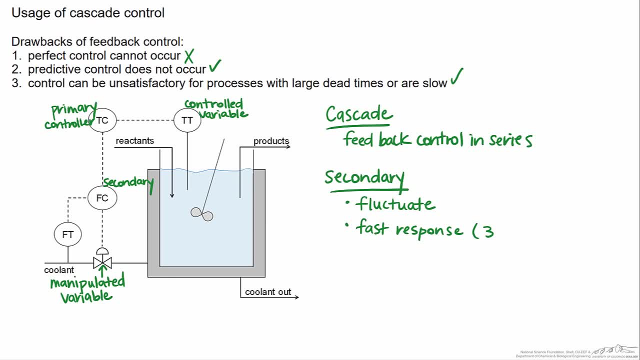 response than the primary loop. A rule of thumb here is about three times faster. where this three times can come from doing some time analysis of the tau value, the time constant, If it's a little less than three times what The issue is? the fact that you now have this counter-balancing between- yes, you're quickening. 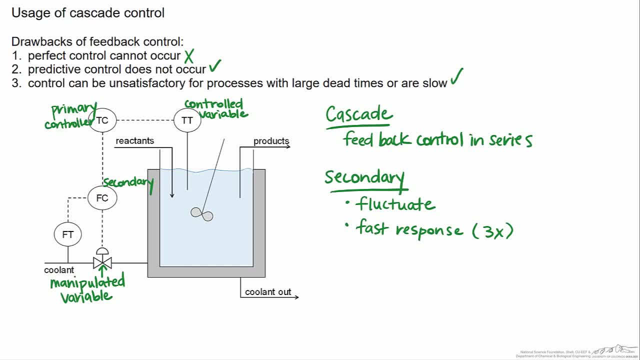 your response. but you've now also introduced new equipment which can have fluctuations or which can break. So therefore, in terms of what is the net gain to the controls overall, it may not be as much as you think. To go back to the issue of why perfect control cannot occur here, the reason why perfect: 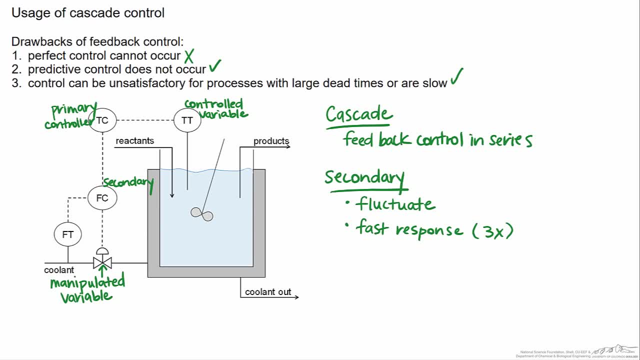 control can't occur here is that there is still a connection here to the primary variable, so in other words the secondary variable. So the primary variable's decision-making process is based on what is going on with the primary variable. so therefore it helps mitigate the idea of the possibility of perfect. 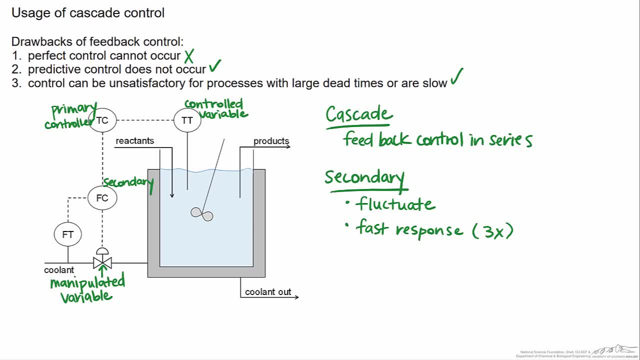 control. So what we'll do here is kind of talk about the loop in a bit more detail. If we see a deviation to the temperature, the controlled variable, the temperature inside the reactor, the temperature controller is going to send a signal to the flow controller saying I: 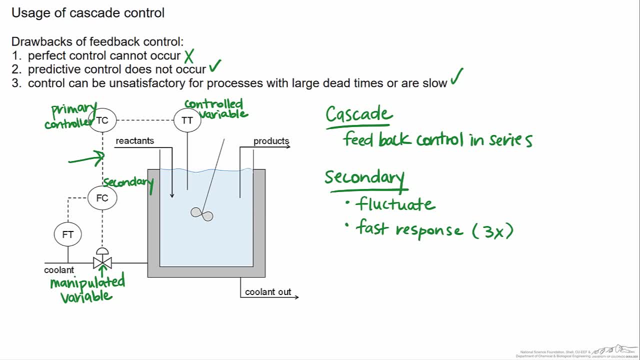 need more or less coolant. So, in other words, what this is really doing is this is going signal here, sent from the temperature controller to the flow controller, is setting a new set point for the secondary controller. So with this new set point, the secondary controller. 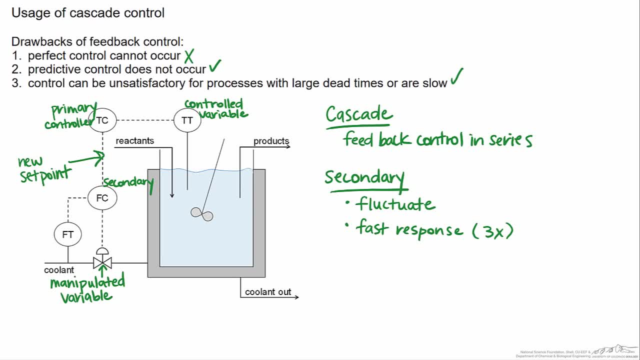 can then take what the new value should be in order to get the desired temperature. compare it to what the flow rate of the coolant actually is. take those two pieces of information together and adjust the valve Additionally. what this can also do is handle adjustments in the flow. 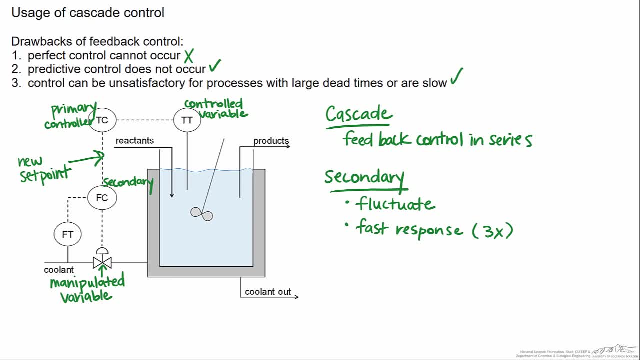 transmitter the flow of the coolant and make those adjustments even if the temperature has not changed Again. this is why the response is quicker than it would have been originally if we just had a pure feedback scheme where the temperature controller was directly connected to the valve. So the question now to ask is: how does this all get represented on a block? 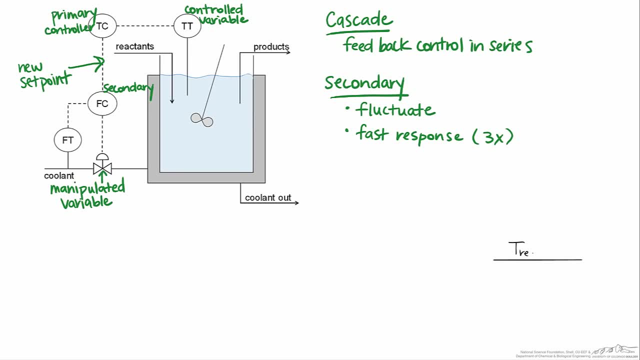 diagram. So to show this, we'll start with our output variable and we'll use the example of the reactor I have here. So therefore, the output variable will give an answer. output here would be the temperature of the reactor. So we'll just follow the sys steps. 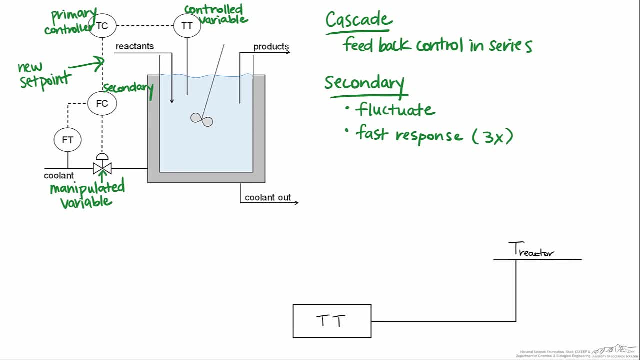 here where, again, this does have a large root in feedback control. so therefore, the temperature of the reactor will then go to the sensor transmitter of the temperature transmitter. From the temperature transmitter it will go to the controller- Remember the fact that the controller has to take in an error, so therefore we need to compare it. 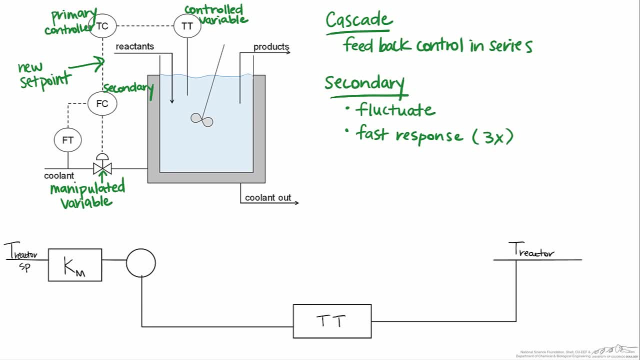 to the set point of the reactor, multiply it by Km in order to get it into appropriate units, and then from there we'll connect it to the controller And in this case, if we follow the arrows here- we're talking here about the temperature controller- We follow. 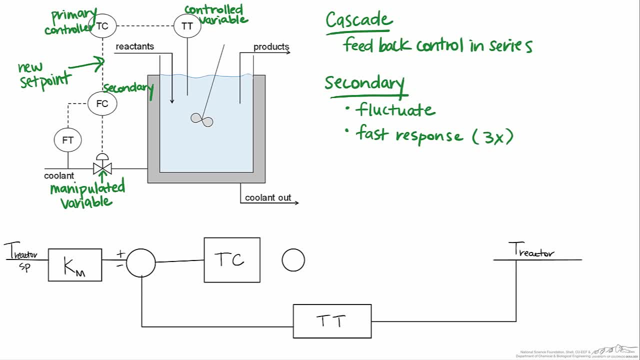 the arrows. further, the temperature controller then sends its information to the flow controller and we note the fact that the flow controller takes in two signals. So we are going to put a summing point here, because we know we're going to need this. So, from the flow controller, 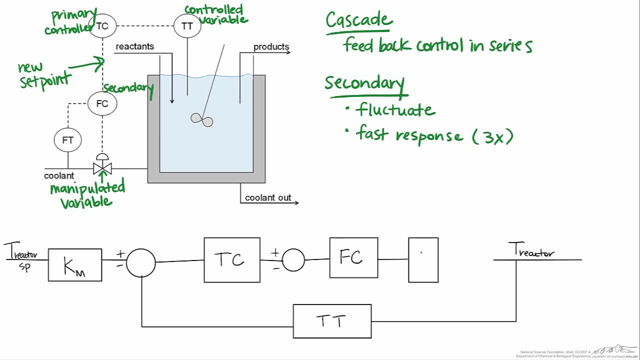 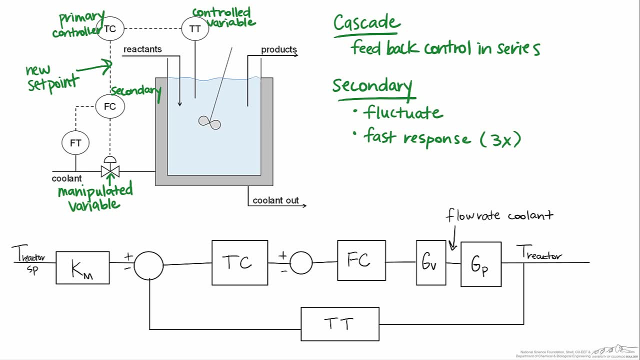 we then send the signal to the valve and then from the valve we then have our process, which is the reactor. So for our case here, what comes out of the valve is the flow rate of the coolant. So because that comes as the flow rate of 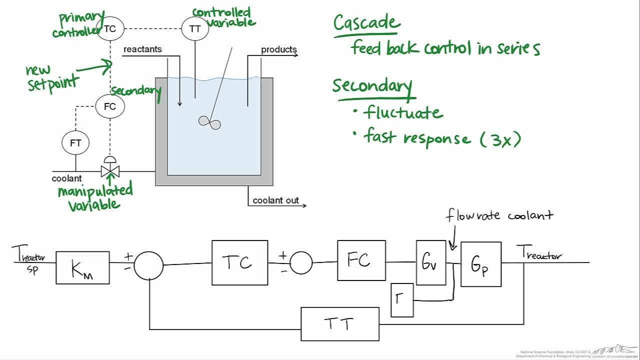 the coolant. we'll draw our cascade part here. This would represent the flow transmitter and we have completed our loops. Therefore, this shows how cascade control represents a nested feedback loop. Because of this nestedness, what this also means is that the secondary 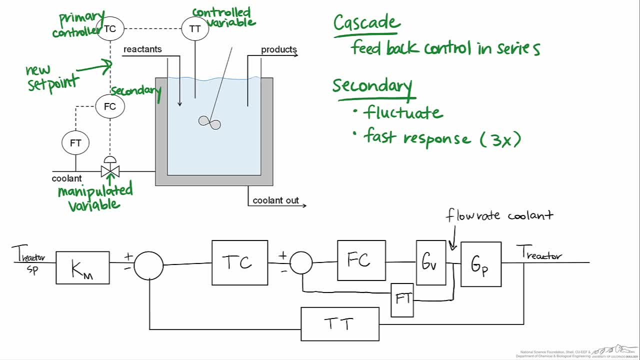 loop impacts the primary loop, and this is most notable with respect to tuning, where, in order to properly tune this control scheme, we also have to take into account the secondary control loop. Generally, when tuning, you tune from the inside out. so therefore, in this, 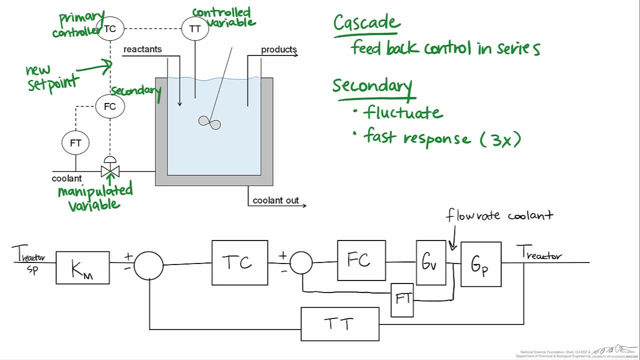 case, we would tune by starting with the secondary loop, then the primary loop. So for the sake of what we are talking about here, this would be the flow loop first, then in the temperature loop. The stability of the process can be greatly influenced by how 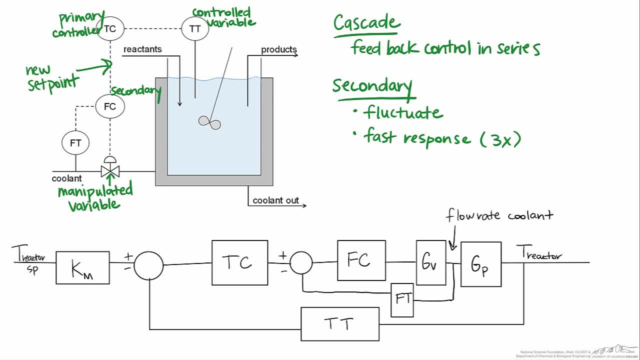 the secondary flow loop has been tuned. So in this screencast we discussed the ideas of cascade control, provided an example and showed how it's implemented, and also discussed the control loop setup for a sample cascade system.